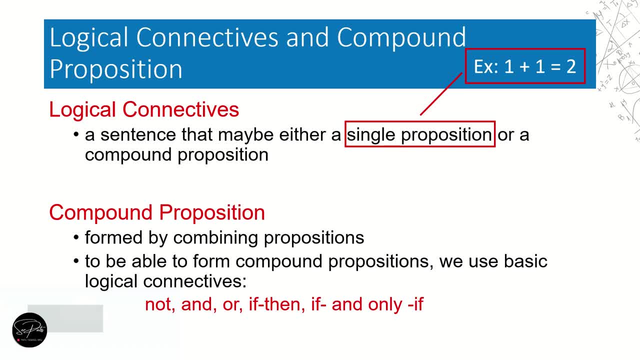 1 plus 1 equals 2.. So that is a single proposition. Pag sinabi namang compound proposition, it can be a combination of propositions. So example we have: 1 plus 1 equals 2.. So that is a single proposition. 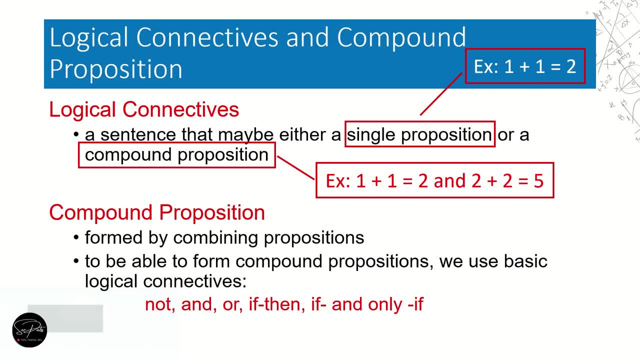 1 equals 2 and 2 plus 2 equals 5.. Huwag nating isipin kung mali yung sagot sa 2 plus 2 equals 5.. So there's no problem with that. So there's no problem whether the answer is correct or not. So if the mathematical sentence relay a false information, there's no problem with that. And compound propositions can be formed by using propositional or logical connectives. So we have example: logical connectives are not and or if, then if and only if. 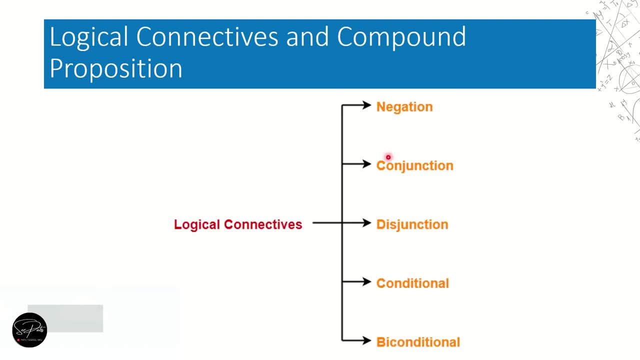 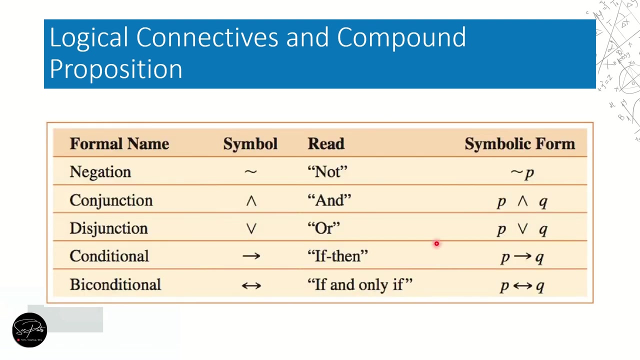 And these are the different types of logical connectives. So we have the negation, the conjunction So negation, so that is the not term that is added to the proposition. Conjunction, So conjunction. we have the and, and this junction is, or Conditional is the if, then, while the biconditional is the if and only if, And these are the symbols that are used in stating a compound proposition. 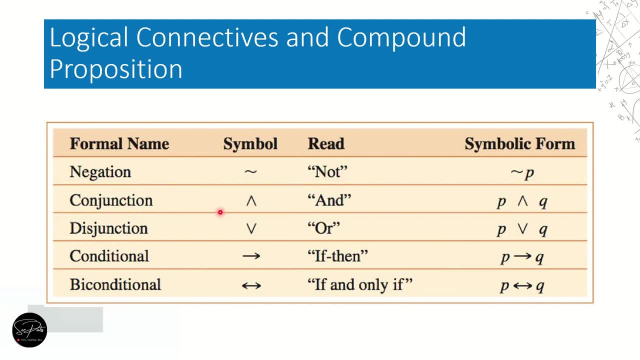 So we have the negation, and the negation is read as not, The conjunction is read as and The disjunction is read as: or And we have the if. then The conditional proposition is read as: if, then, And the biconditional proposition is known to be as the if, and only if. 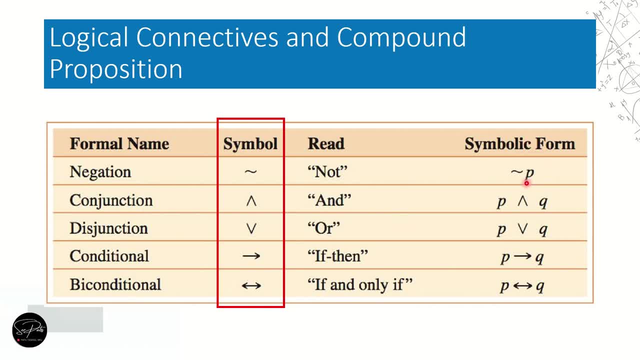 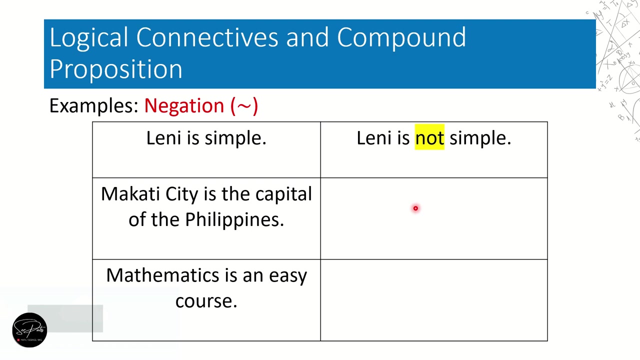 So kung babasahin natin yung symbolic form, we have not P, P and Q, P or Q. If P, then Q, P, if and only if Q. Examples of negation, of negation. So we have here example: proposition is: len is simple and the negation will be, len is not simple. 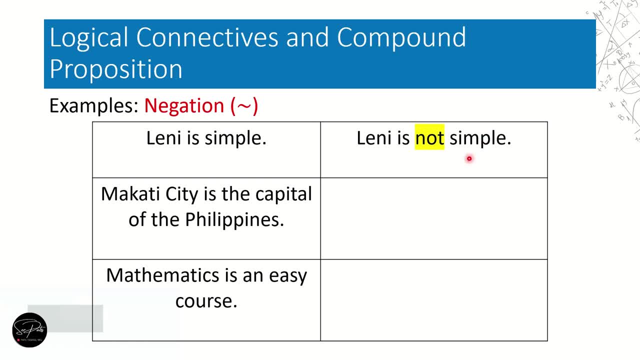 So kung baga dinuktung lang natin yung term na not, in order for the statement to be converted into false proposition, Makati City is the capital of the Philippines, Ang kanyang negation will be: Makati City is not the capital of the Philippines. 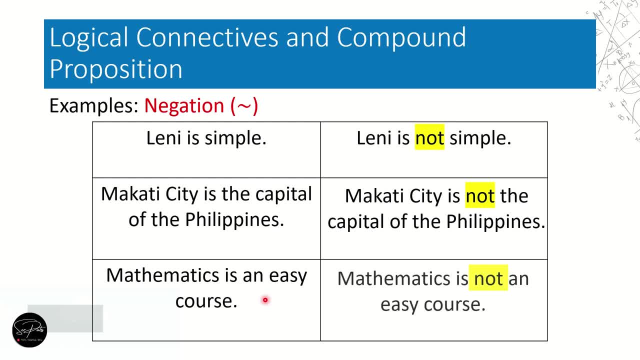 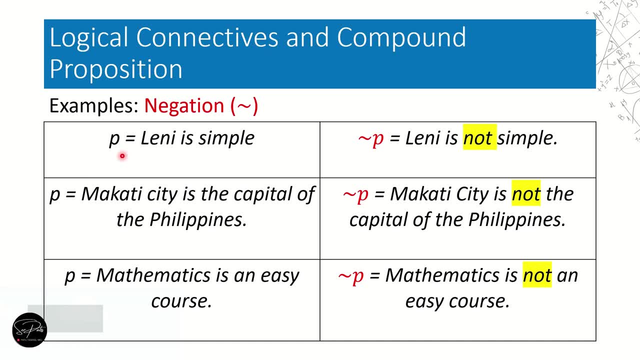 And third, we have: mathematics is an easy course and the negation will be. mathematics is not an easy course. And if we will convert the proposition into variables? so example we have: P is equals to len is simple. The negation of P or not P len is not simple. 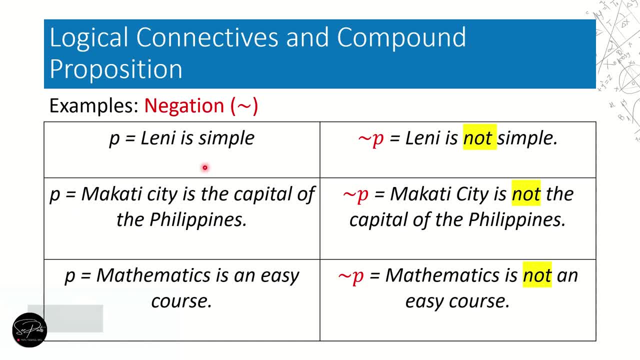 So kung baga yung mga statement natin, kanina for the proposition, binigyan lang natin ng variable P To represent the proposition. So we have here: P is equals to. len is simple, not P. len is not simple. 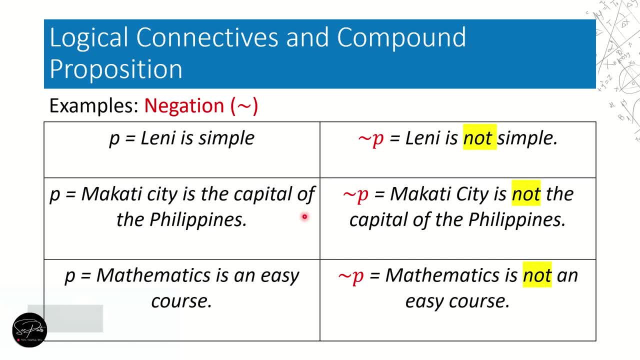 Then P is equal to Makati. City is the capital of the Philippines, not P. Makati is not the capital of the Philippines. Then P is equal to mathematics is an easy course, not P is equal to. mathematics is not an easy course. 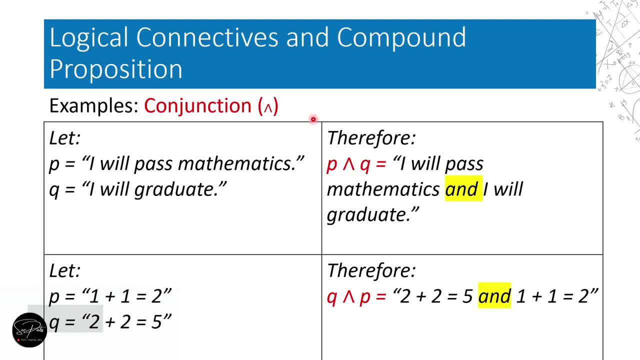 Then we have conjunction. So second of the type of logical proposition is the conjunction And conjunction is So. let us end. Example: we have here our proposition. So we have P is equal to I will pass the mathematics And letter Q will be I will graduate. 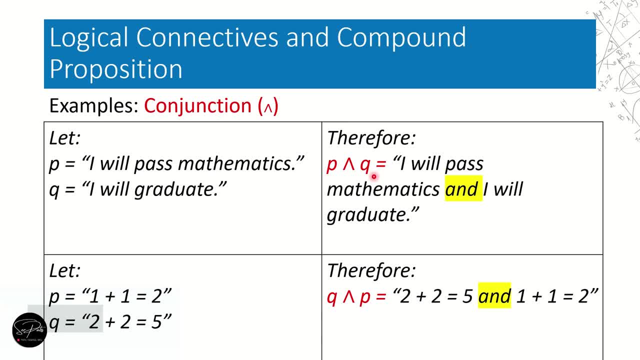 Therefore, pag nagkaroon tayo ng P and Q for our logical proposition, that will be stated in English sentence, as I will pass mathematics and I will graduate. So we have P and Q, So yung dalawang statement natin, kinumbay lang natin using the conjunction and: 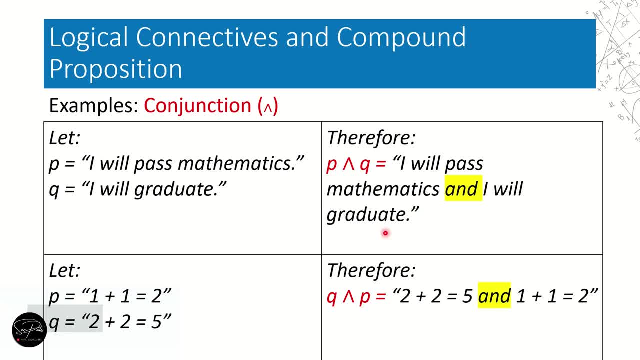 I will pass mathematics And I will graduate For second example. so we have one plus one equals two. two plus two equals five Again, so there's no problem whether the statement is correct or not. Therefore Q and T, So nauna yung letter Q natin, So ang value ng letter Q natin will be two plus two equals five. 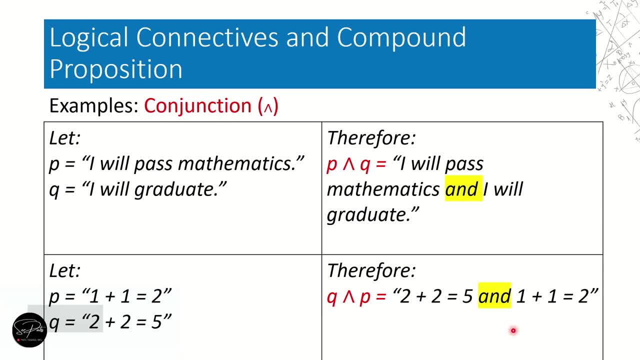 So that will be the first proposition, And connected by the conjunction. and one plus one equals two, So our conjunction will be: two plus two equals five, And one plus one equals two, which is equivalent to Q and P Disjunction, or, or: 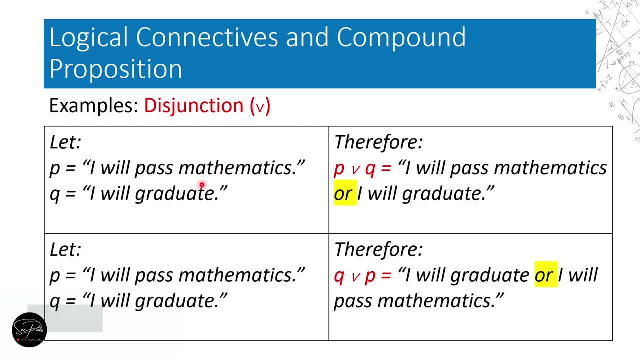 So ito naman ay binabasa na. or We have the same example here. I will pass: mathematics is P, Then Q is I will graduate. So we have P or Q, So the English equivalent will be: I will pass mathematics or I will graduate. 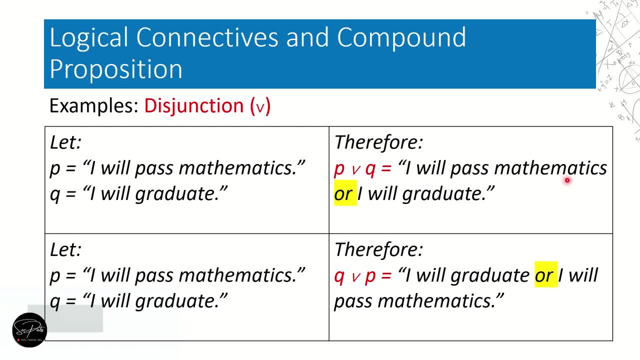 P or Q. I will pass mathematics- That is the first proposition, which is the equivalent of P- And I will graduate. That is the second proposition, which is the equivalent of Q, And our logical connective will be: or P and Q. 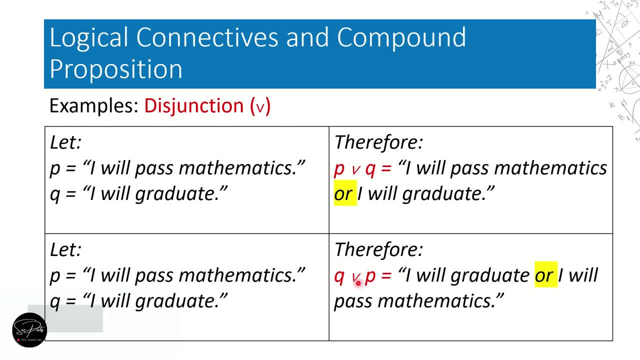 I will pass mathematics for P. I will graduate for Q. So binaligtad naman natin Q or P. So if Q will be the first variable, so we will have the value of Q as our first proposition. I will graduate or I will pass mathematics. 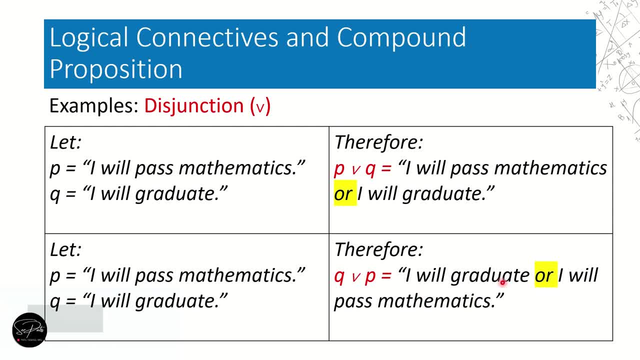 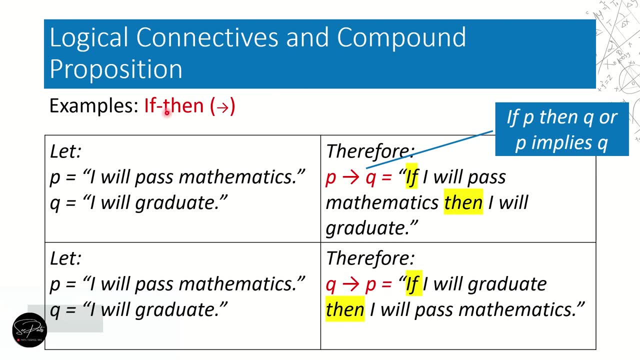 So sa pangalawang example natin, na una yung I will graduate, kasi sa ating given na una yung Q And sumunod yung P. So sumunod yung I will pass mathematics. And for our next type of proposition, of compound proposition using logical connectives, we have the if-then. 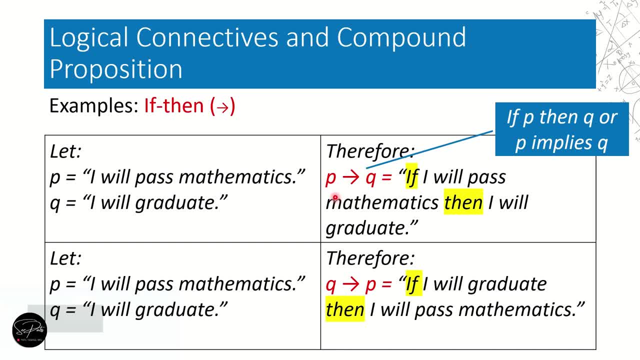 Etong arrow na to nag-represento ng if-then So example. here we have if P then Q, So binabasa natin siyang: if P then Q, Or P implies Q, Pwede na naman yun. 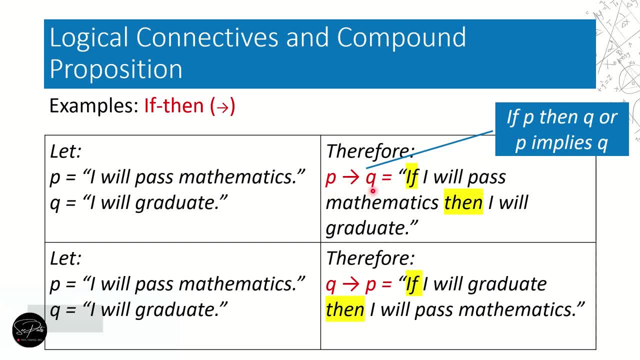 So na una, yung variable P. natin then sumunod yung ating variable Q And P is equivalent to I will pass the mathematics And Q is equivalent to I will graduate. So that will be: if P, then Q is equal to if I will pass mathematics, then I will graduate. 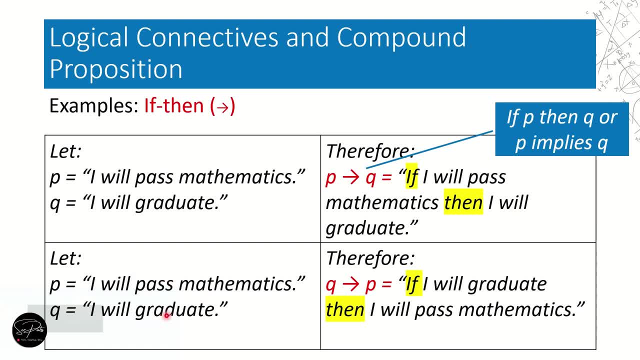 Second example: we have the same statement here, same proposition here: I will pass mathematics for P, I will graduate for Q, Then ang given natin dito. So if Q then P, So binalik natin. So that will be: if Q then P. 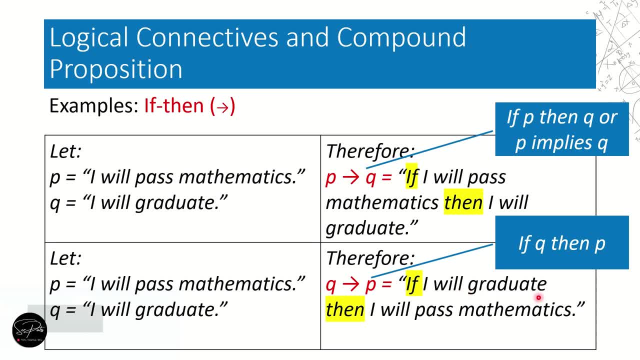 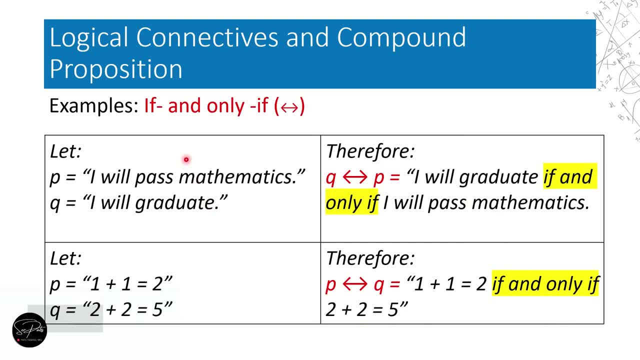 So, mauna, yung ating Q statement. So that will be, if I will graduate, then I will pass mathematics. And next proposition type, next compound proposition type using logical connectives, we have the if and only if, So that will be represented by a double-headed arrow. 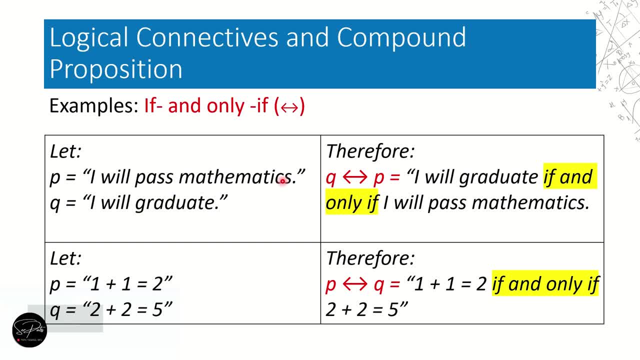 Example: same, Same, So I will pass mathematics. Q is equal to I will graduate. So therefore this is read as Q, if and only if P. So yung equivalent ng letter Q natin will be I will graduate, Na una, yung letter Q. 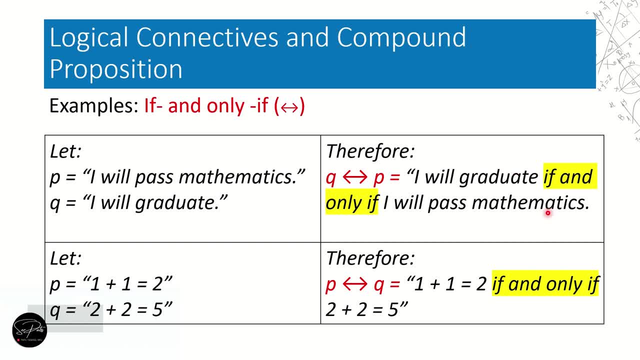 I will graduate if, and only if, I will pass mathematics. Okay, then an example: number: 2.. 1 plus 1 equals 2.. 2 plus 2 equals 5.. So again reminder, Huwag nyong intindihin kung tama o mali yung sagot natin. 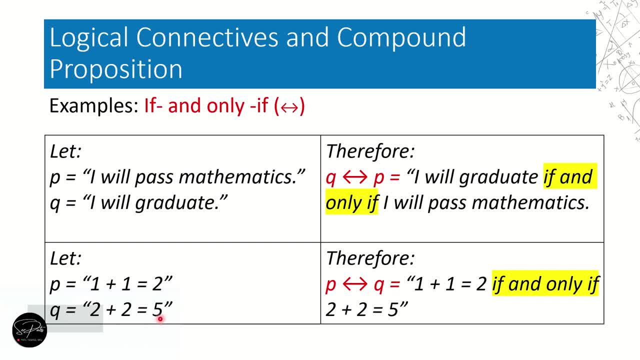 Hindi natin pinag-uusapan yung tama O mali, yung ating answer, Because sabi natin sa definition kanina proposition can be true, it can be false, but not both. Therefore P, if and only if Q. 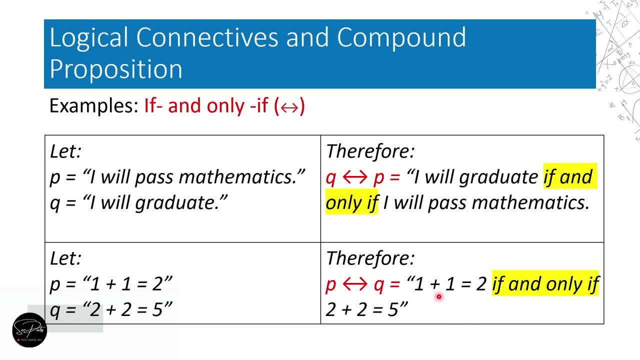 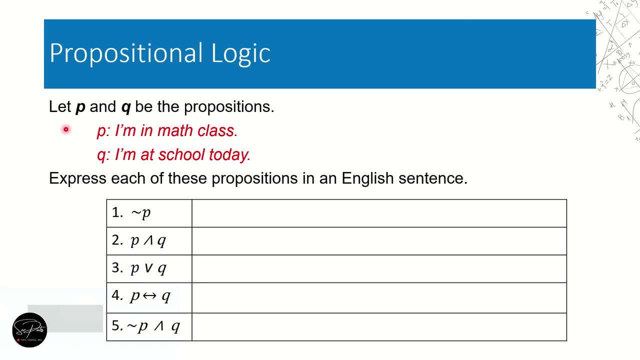 So nauna yung ating letter P, So that will be 1 plus 1 equals 2.. If, and only if, So unod yung ating Q: 2 plus 2 equals 5.. And let's have more examples here. 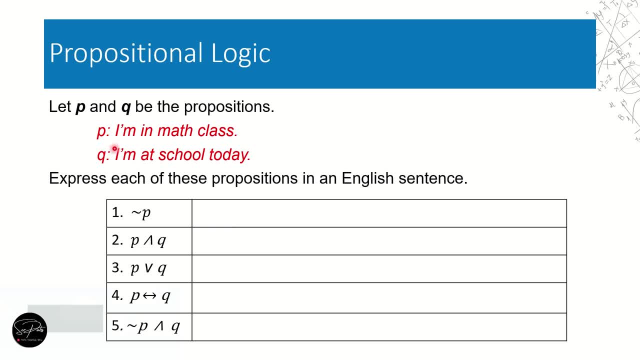 So we have here, let P and Q be the propositions: P I'm in math class And Q I'm at school today. So instruction: We have expressed each of these propositions in an English sentence. So bago natin express, basahin muna natin yung mga examples natin. 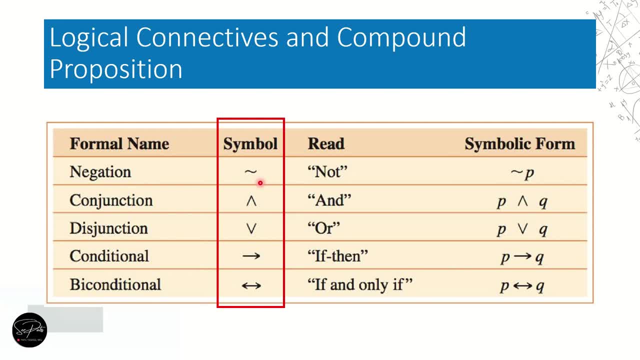 So we have not P Review natin yung ating mga symbols. So the symbol for negation or not, Symbol for and Symbol for or If, then If and only if, Yan yung mga dapat natin tandaan na logical connectives. 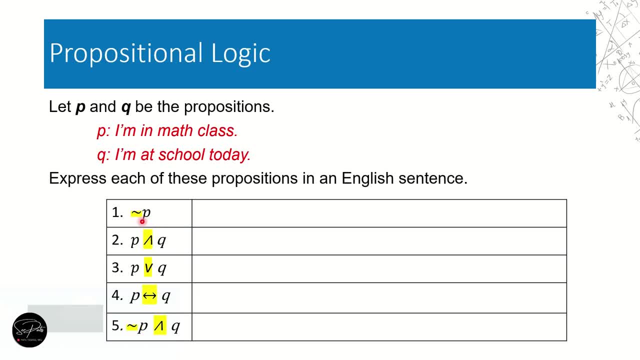 Okay, so let's go back here. So we have not P- number 1.. Number 2, P and Q- Number 3. Number 4, we have P if, and only if, Q And for number 5, so that will be not P and Q. 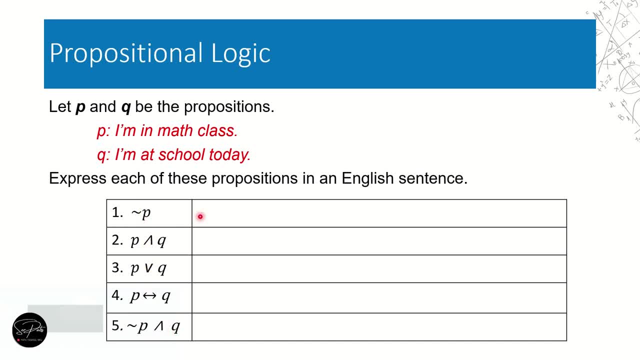 Okay, so let's try now to convert the following propositions into an English sentence. So based on our given proposition, So not P ang letter P natin. I'm in math class, So therefore we'll just insert the word not dun sa ating proposition. 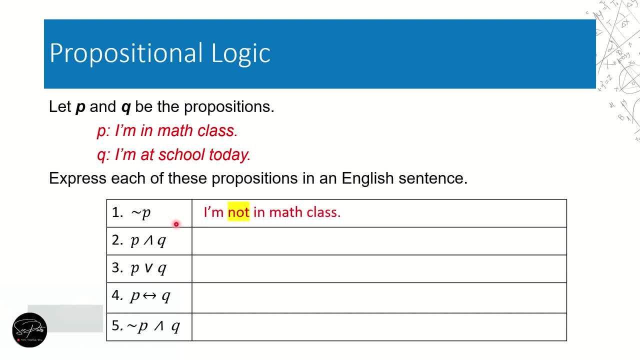 So that would be: I'm not in math class. Then, second, we have P and Q. So we have P and Q, So let's combine the two propositions using: and. So we have here: I'm in math class and I'm at school today. 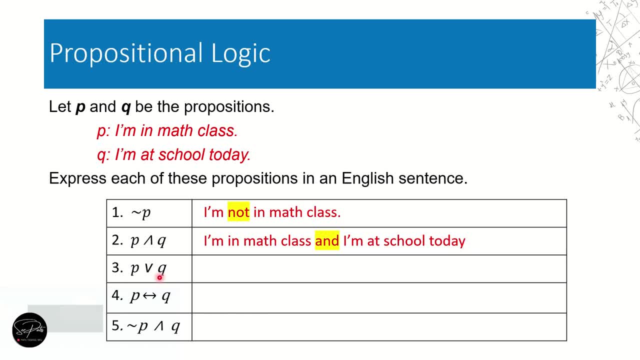 And third, we have P or Q. Okay, we have P or Q, So that will be: I'm in math class or I'm at school today. For the fourth compound propositions, we have here P, P And only if Q. 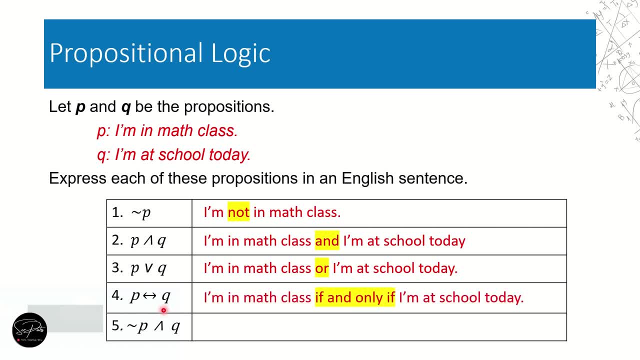 So that will be equivalent to I'm in math class. if, and only if, I'm at school today, Then for number 5, kung diting na natin si number 5, alos pinaeksama siya na number 1 saka number 2.. 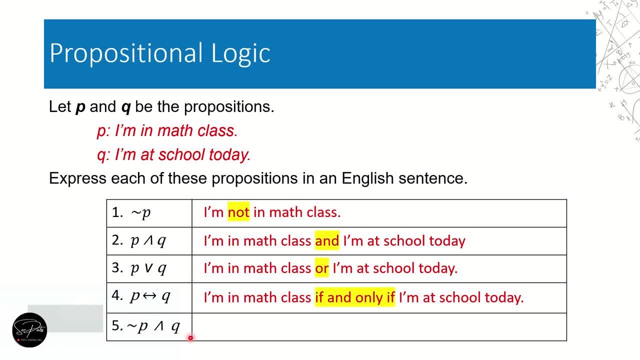 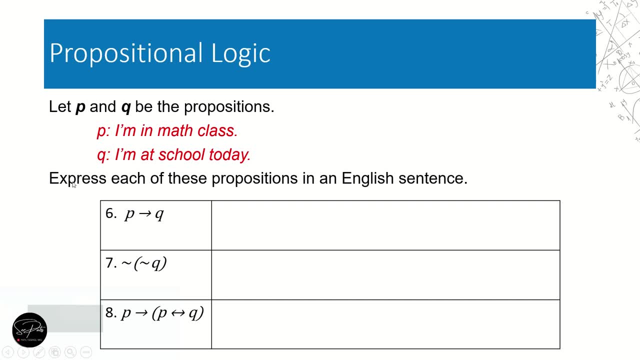 So meron tayong negation for letter P, So not P and Q. So we have here: I'm not in math class and I'm at school today And let's go back here. So again we have here: let P and Q be the proposition. 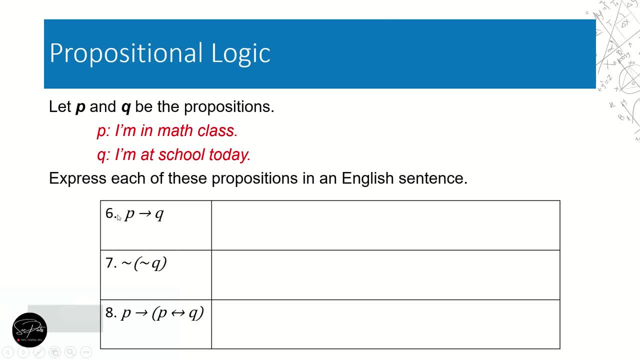 So: P- I'm in math class, Q- I'm at school. I'm at school today. So ang ating number 6 ay. if P, then Q. So that will be equivalent to: if I'm in math class, then I'm at school today. 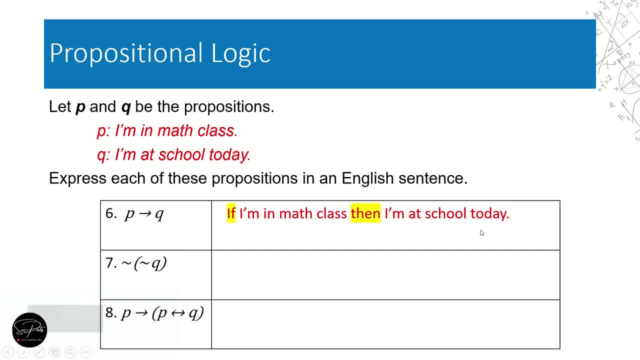 So if P I'm in math class, then Q I'm at school today, Then for number 7, so meron tayong negation of, not Q, So kailangan ko natin tingnan yung ating truth table. 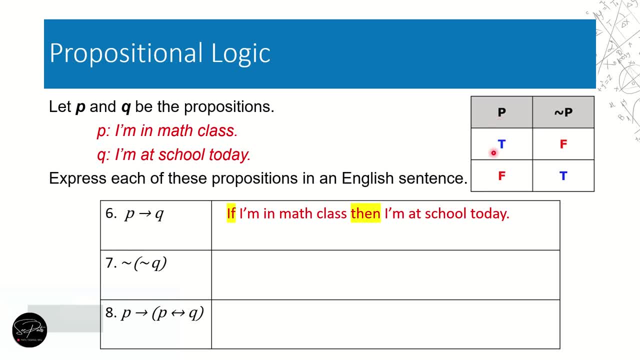 So ganito yung pagtingin ng truth table natin: Kapag daw tama yung proposition, if the proposition is already true, then we have to look at the truth table. So if the proposition is already true, yung ating negation will be false. 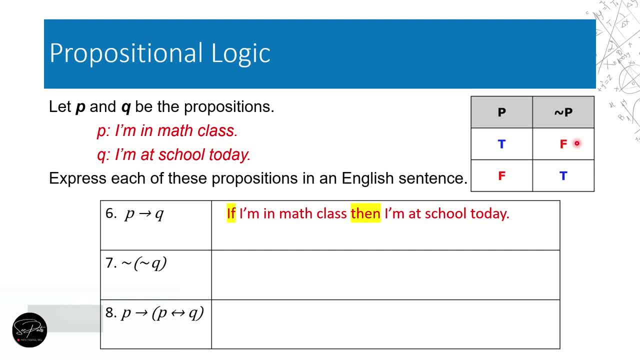 Mamamali yung statement ng ating, not P, For example, Manila is the capital of the Philippines, Tama yun. So ang negation natin, Manila is not the capital of the Philippines, So that will be false. Okay, kapag mali na yung ating proposition, so ang negation nya magiging tama. 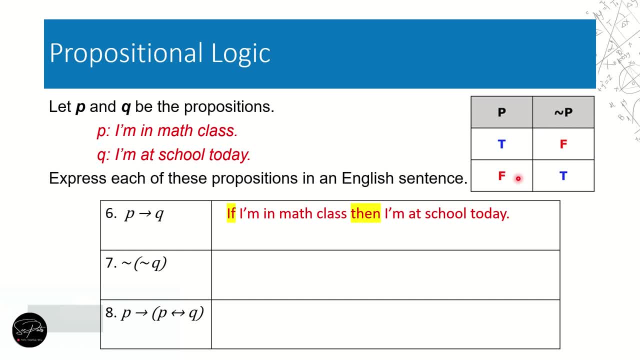 So alimbawa, Manila is not the capital of the Philippines. Ang negation natin hindi pwedeng Manila is not not Diba, hindi natin pwedeng sabihin na Manila is not not the capital. Iko-convert lang natin sya ng true. 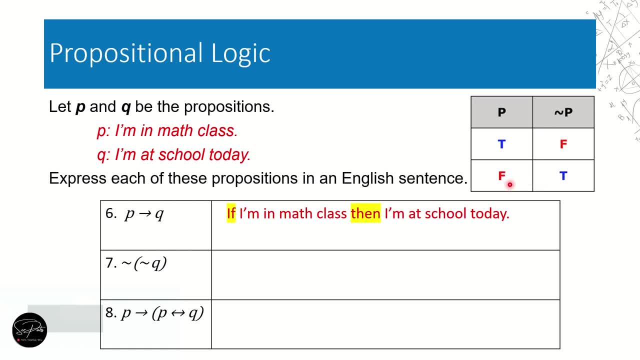 So parang ang ating proposition: Manila is not the capital of the Philippines, So tanggalin natin yung not That will be the negation. So Manila is the capital of the Philippines, So ganun yung mangyari. 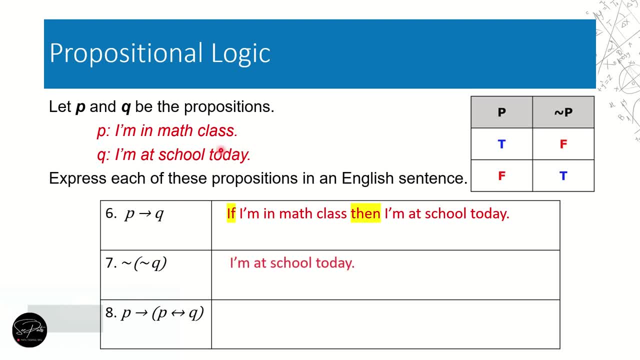 So dapat dito: ang ating negation of Q ay equivalent to: I'm not at school today. Yun ang ating, not Q. And then nagmeron pa syang negation sa labas ng parentheses, So therefore parang maka-cancel out lang yung dalawang negative. 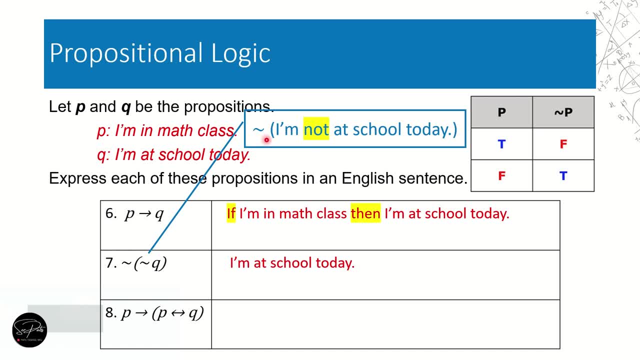 So yung dalawang negation natin. So ang magiging answer natin will be: I'm at school today, So nawala yung ating not Kasi nga mali na yung ating negation. 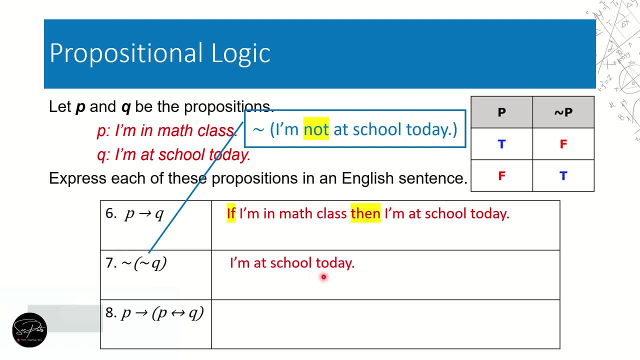 So mali ng mali magiging tama. So I'm at school today And then number 8, so we have If P, then Q, P, if and only if Q. So ang ating if P. 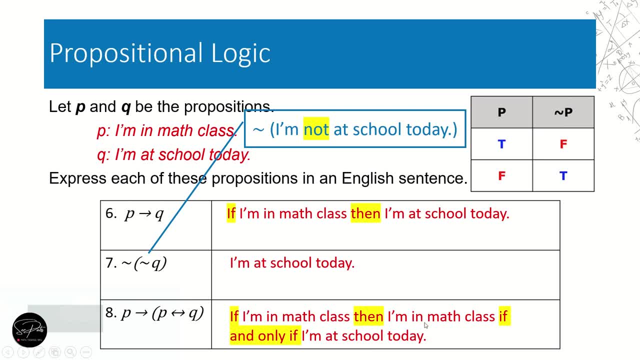 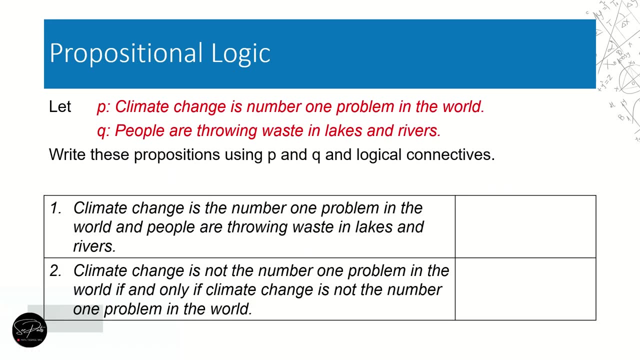 if I'm in math class, then I'm in math class if, and only if, I'm at school today. So ganyan yung paggamit ng logical connectives in a compound propositions. Then let's have another example here. 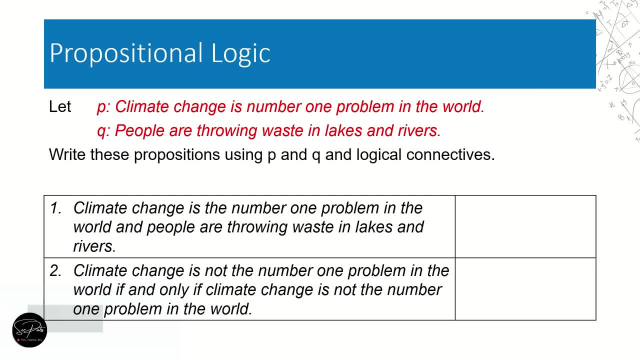 So babalik ta rin naman natin nasa English sentence yung ating compound propositions, Sililipat naman natin ang mathematical statement or propositional logic statement. So let P. climate change is the number one problem in the world. 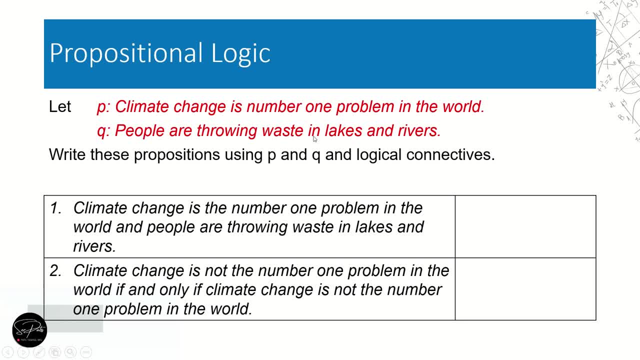 Then people are throwing waste in lakes and rivers. ang ating letter Q, So write these propositions using P and Q and logical connectives. So yung first statement natin dito: climate change is the number one problem in the world. So that will be P. 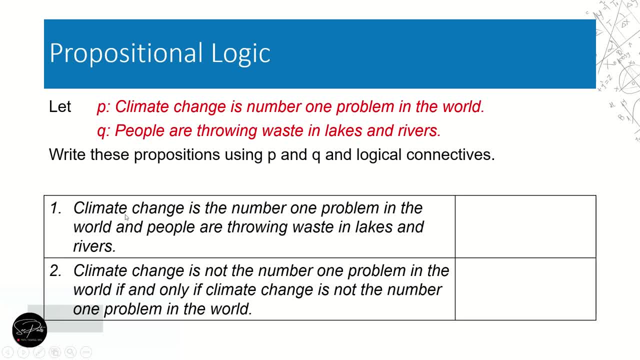 And then connected by N. So people are throwing waste in lakes and rivers. So therefore yung number one natin is a type of conjunction, So naga represent sya ng conjunction. So we will just have the conjunction symbol in between P and Q. 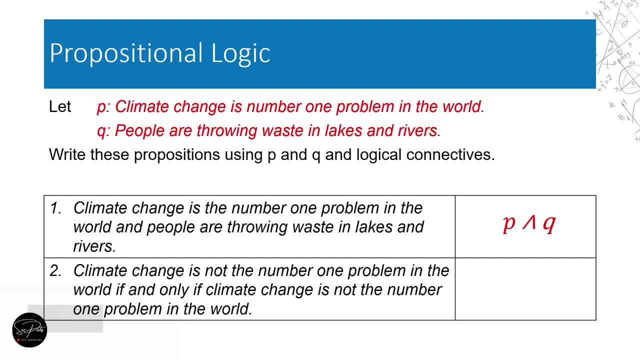 And second, climate change is not the number one problem in the world. So inenegate natin yung ating letter P, Lalagyan natin sya ng not symbol or negation symbol, And then in between meron tayong if and only if. 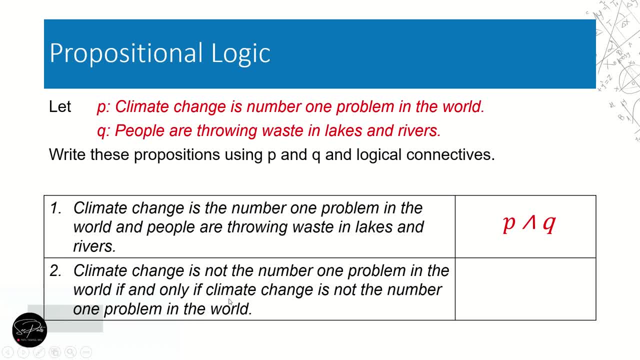 So ang gagamitin naman natin doon ay double-headed arrow. If, and only if, climate change is not, Meron na naman tayong not dito. So meron tayong negation ng P. Nayari sa ating symbol ay negation of P. 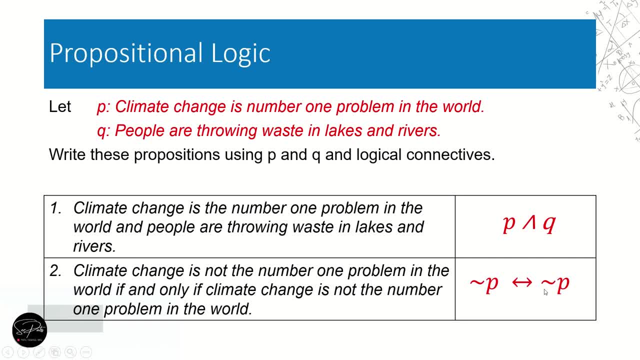 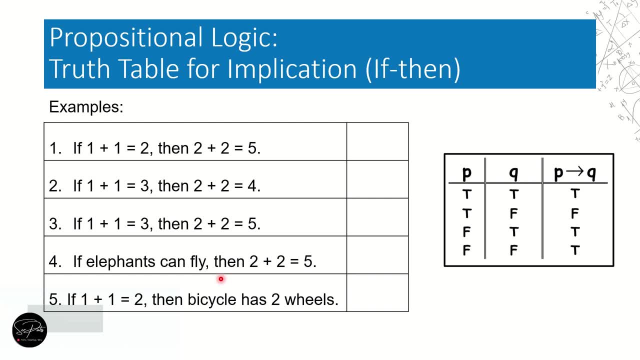 If and only if. negation of P, So not P, if and only if not P. And then let's apply the if-then truth table. So if-then truth table naman tayo, Kanina, binigay natin yung truth table ng ating not. 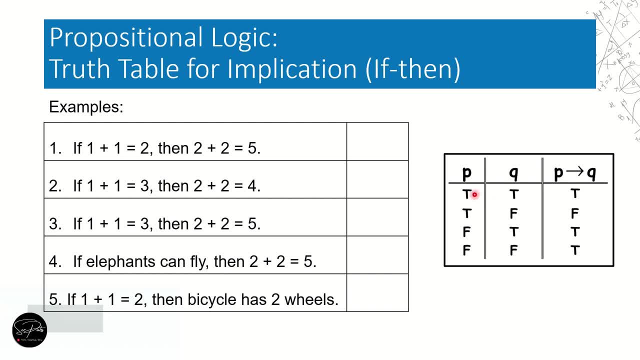 So ngayon, if-then? So, kung ang letter P daw natin ay true, tama din yung ating letter Q. So if both are true, the compound proposition is also true. And then, pangalawa, kung true, yung ating letter P. 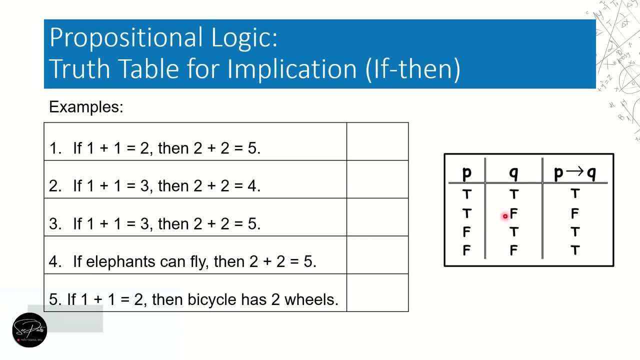 false yung ating letter Q, So P is true, Q is false. The compound proposition, the if-then statement, will be false Later on i-apply natin dito Then F, T, So mali yung P. 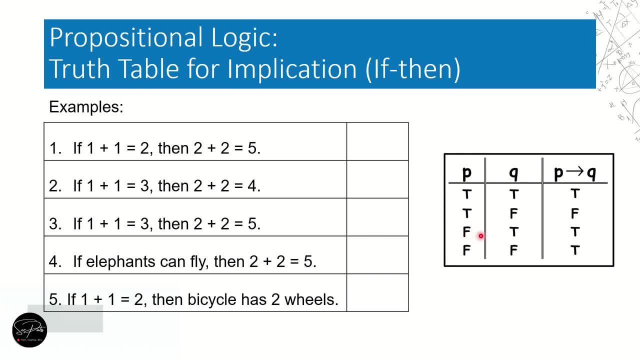 False yung P natin And then true yung ating Q, So the compound proposition will be true. Kung parang naman silang false magiging true tayo. E parang yung kanina diba, sabi natin, kapag ka mali. 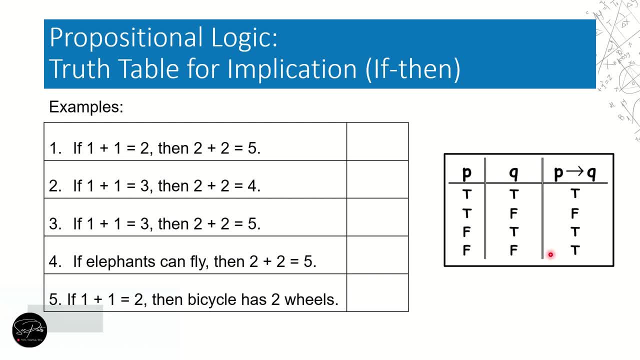 yung letter P natin, yung ating negation of P will be true. So yung kanyang kabaliktaran magiging true, siya, Okay. so example: 1 plus 1 equals 2.. Then 2 plus 2 equals 5.. 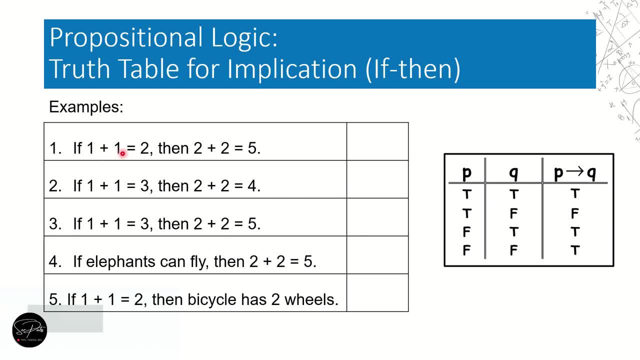 So yung first statement natin is true, Kasi 1 plus 1 equals 2.. So that is true. Yung second statement natin ay false. So tingin ka lang sa ating true table. So we have true and false. 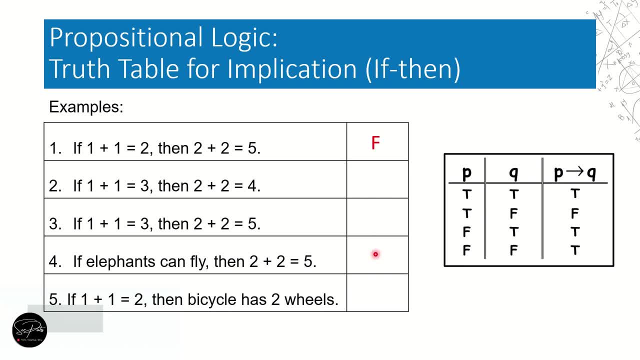 So ang ating if-then statement will become false. Tama yung una, mali yung pangalawa. Tama yung una, mali yung pangalawa. The statement will be mali or false. Number 2, mali. 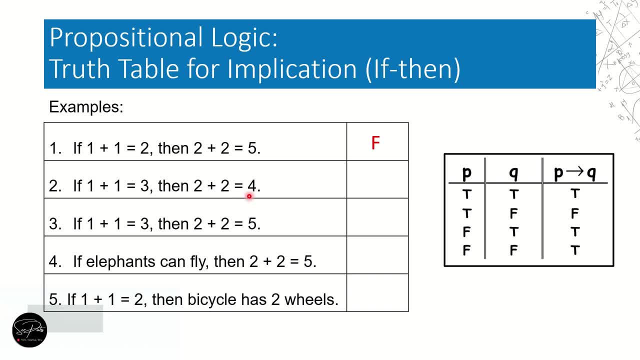 1 plus 1 equals 3. False: 2 plus 2 equals 4. True. So mali tama Hanapin sa true table. Ito yun yung pangatlo. False yung P. 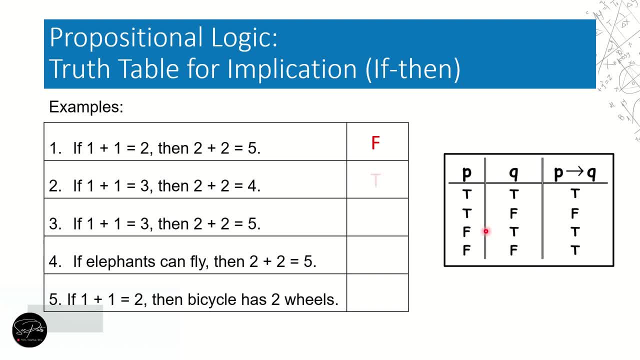 Yung, letter Q ay true, So therefore the statement will be true Again: mali tama, Mali tama tama. So that will be true. Number 3, we have: 1 plus 1 equals 3..